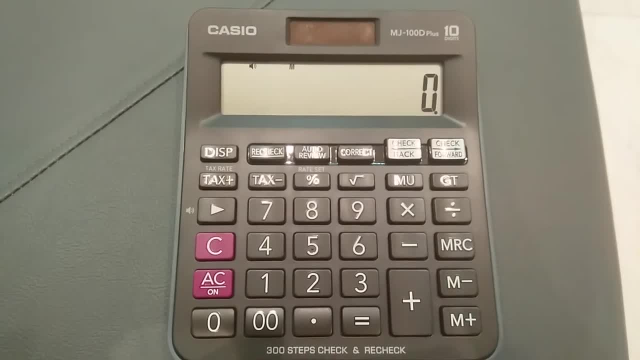 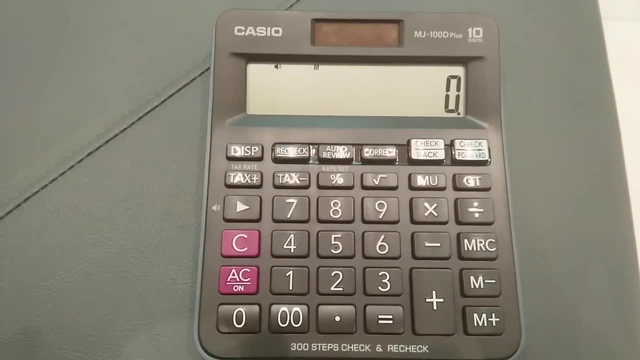 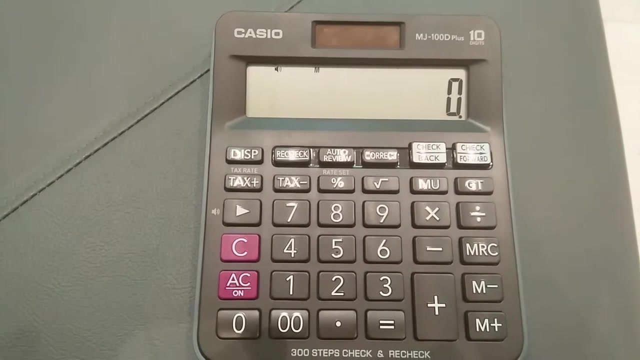 hi guys, I hope you are doing very well and today I'm going to show you how you guys can do the repeated addition and repeated multiplication in your Casio calculator or any calculator, using this simple technique, guys. so, guys, it's very easy. if you want to do the repeated addition, I will show you how you guys. 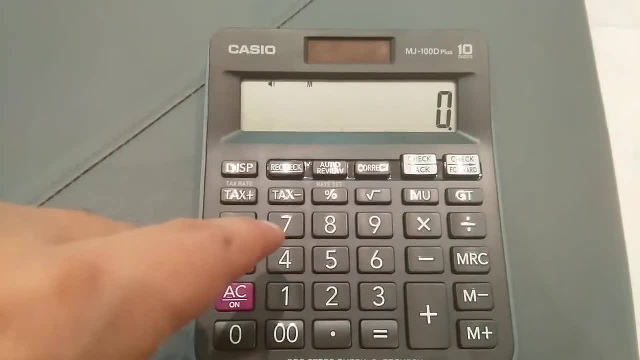 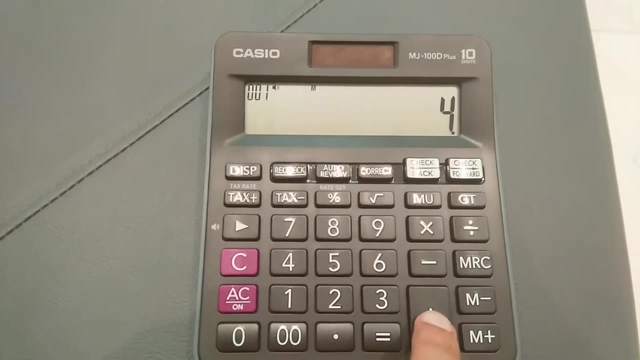 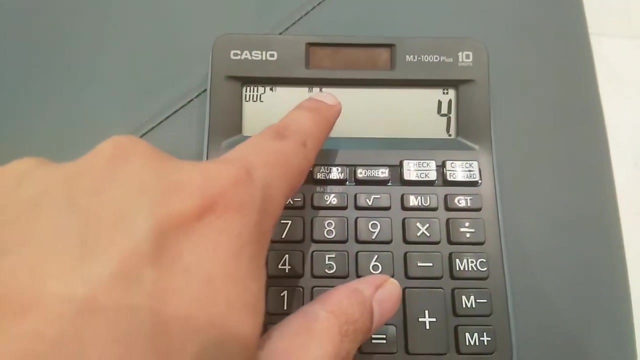 can do it. so first you have to press whatever value you want to do the repeated addition. for example, I want to do four, I want to repeated addition, so I have to press this plus button two times one and this is two. so, guys, when you press this two, there is a sign like K is coming here, and then you have to press. 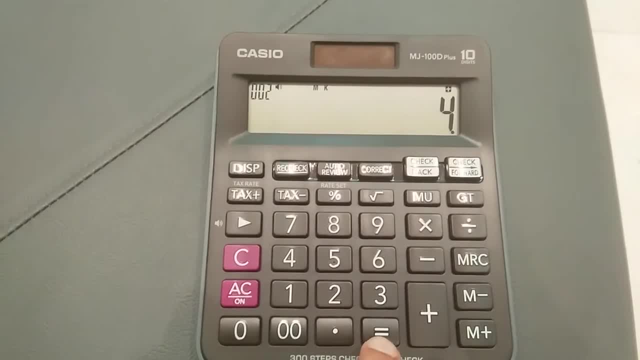 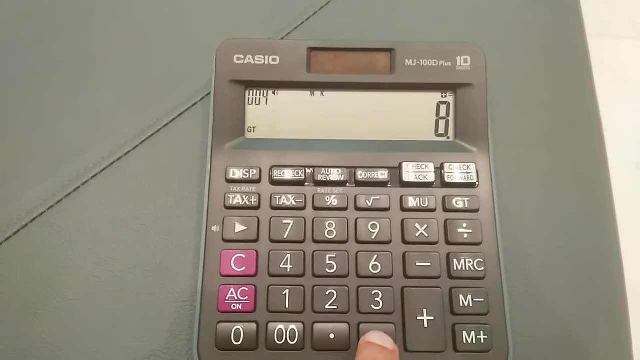 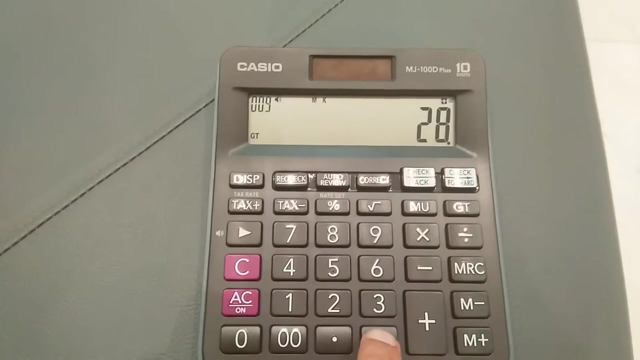 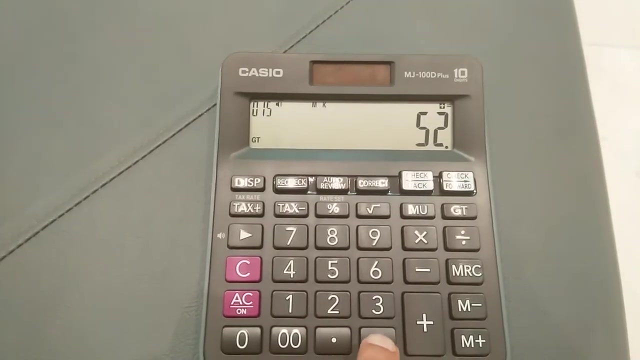 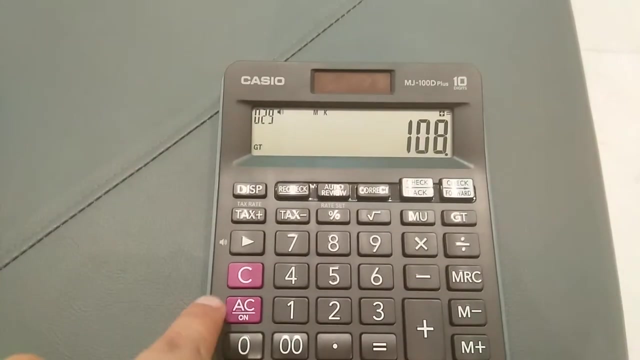 this equal button. so when you keep pressing this equal button it will automatically repeat it, start repeated addition 8, again 12, as you guys can see. it's repeatedly addition 4 and into the total values guys you can see here. so when I keep pressing this button it will start a repeated addition. you can do. 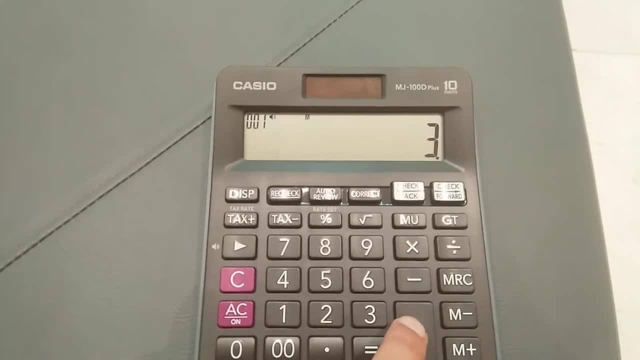 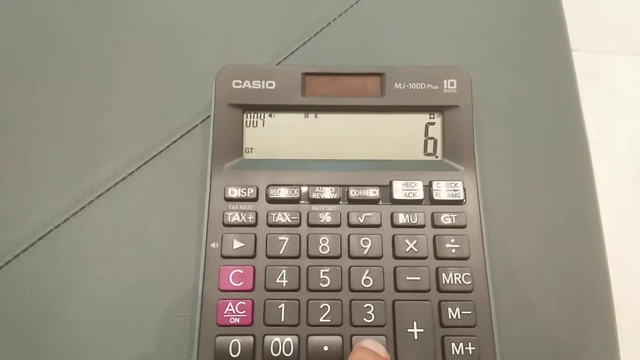 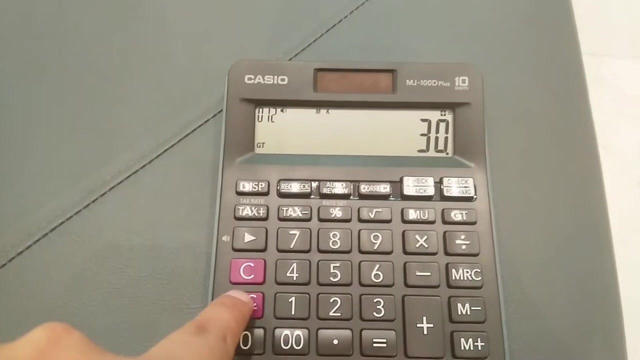 this with any value. for example, you want to do three here and then you have to press plus, two times plus plus, so it start repeated addition. now press starting equal button, six, nine, twelve. so, guys, as you can see, it is keep repeated addition. so now the second thing I want to introduce you. 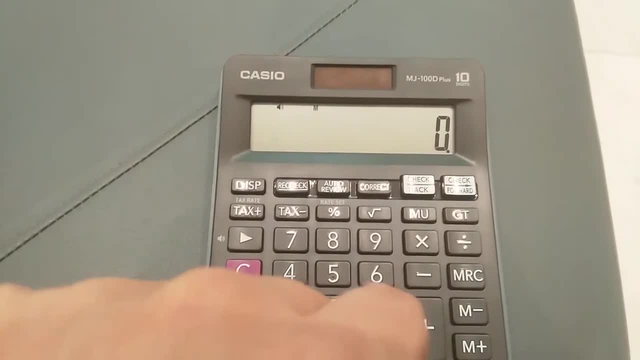 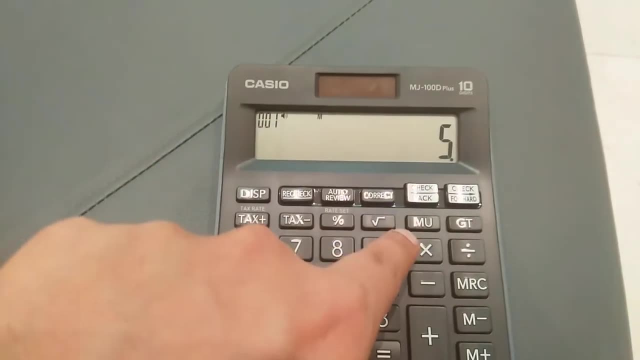 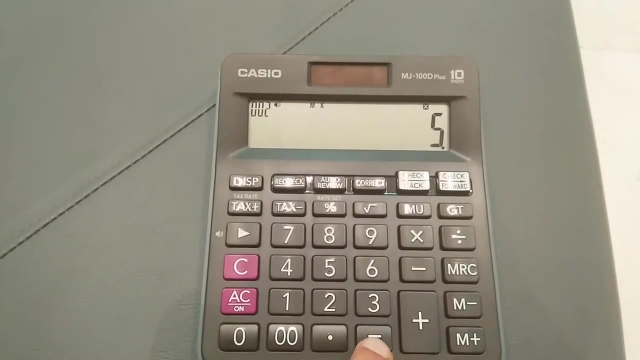 is repeated multiplication. so what you have to do if you have any value like, let's say, you have a five and you want to do repeated multiplication with the five, so simply you have to press this multiplication button two times. so when you press it two times and then after start using the same equal button, so five. 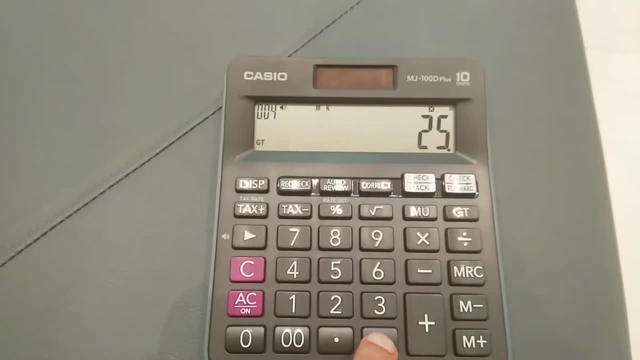 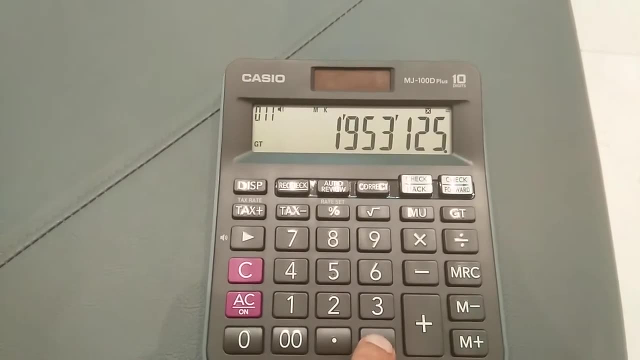 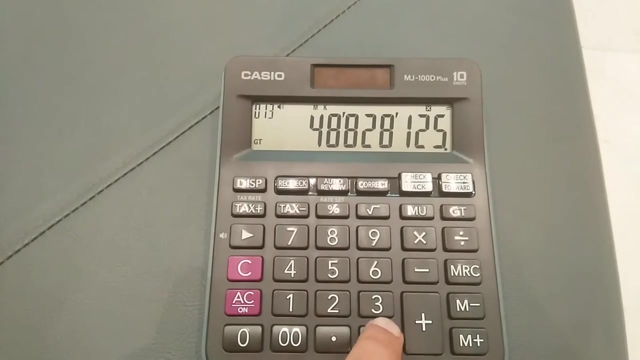 multiplied by five is equal to twenty five. now it start multiply five with these value guys. you can see here so automatically. you can see it start repeated multiplication and you can see here the value increases as we repeatedly multiply the value with the five guys. so, guys, I hope you get the 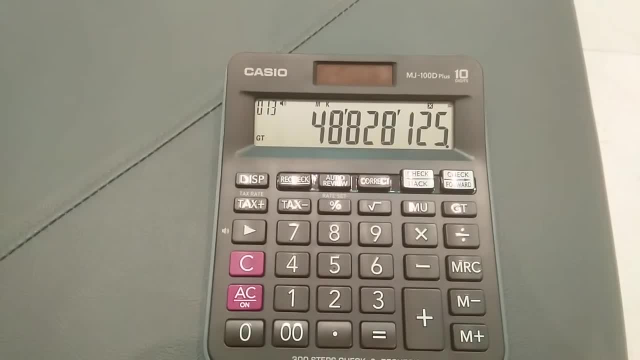 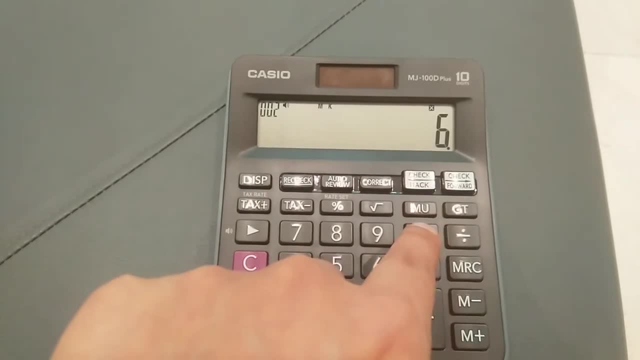 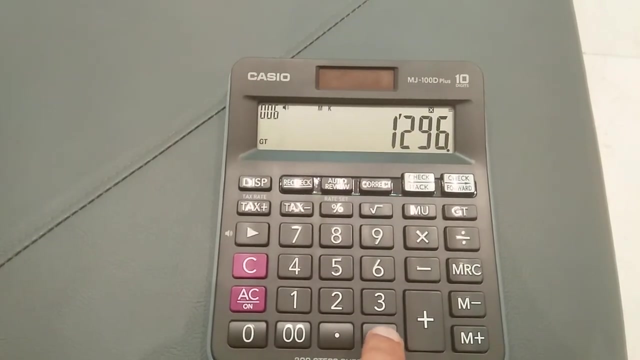 whole idea of this repeated multiplication and I hope you like my video. you can use any other number, six for example, and you want to do repeated multiplication with six. press, multiply two times and then equal to start. equal six multiplied by six, thirty six, and you can see here it's keep multiply its own and becoming a repeated